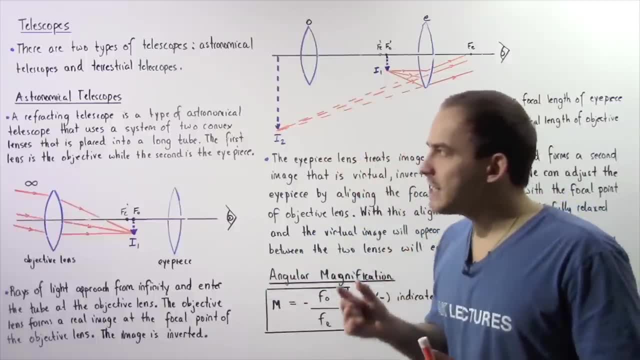 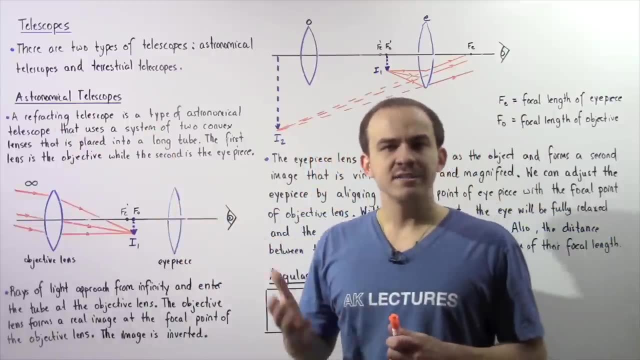 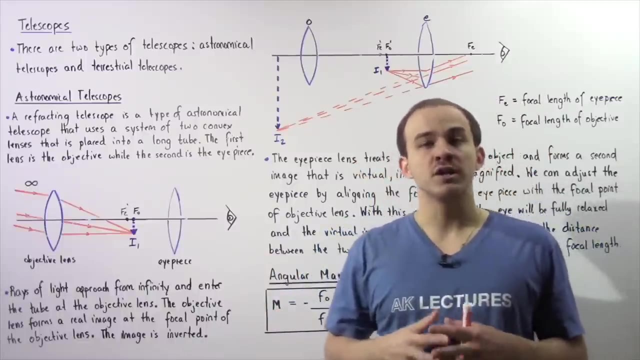 Now in this lecture we're going to discuss a specific type of astronomical telescope known as a refracting telescope. So a refracting telescope is a type of astronomical telescope that uses a system of two convex or interactive telescopes. So, as you can see here, a refracting telescope is a type of astronomical telescope that uses a system of two convex or 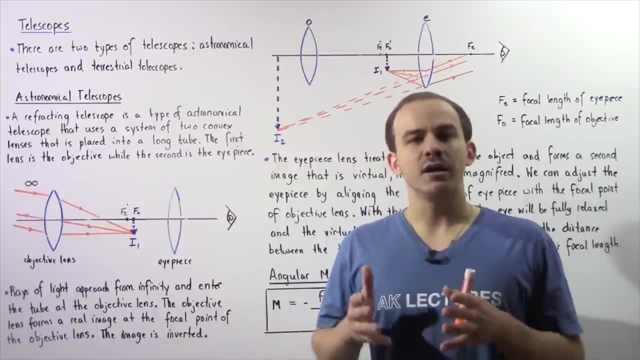 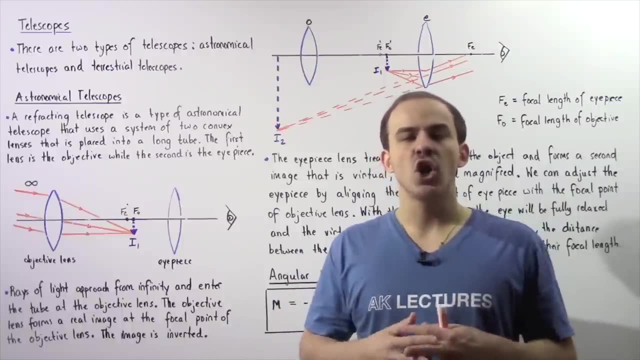 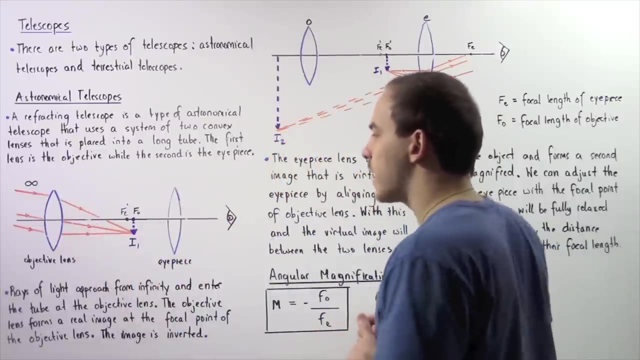 converging lenses that are placed inside a long tube. Now the first lens is known as the objective lens and the second lens is known as the eyepiece lens. So let's see exactly what we mean by looking at the following diagram. So let's suppose we have a long tube Lens number one, a convex lens. 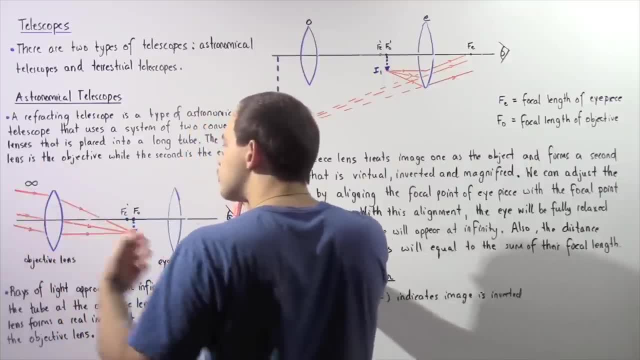 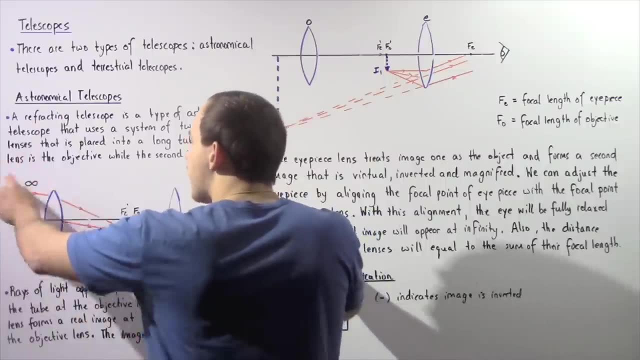 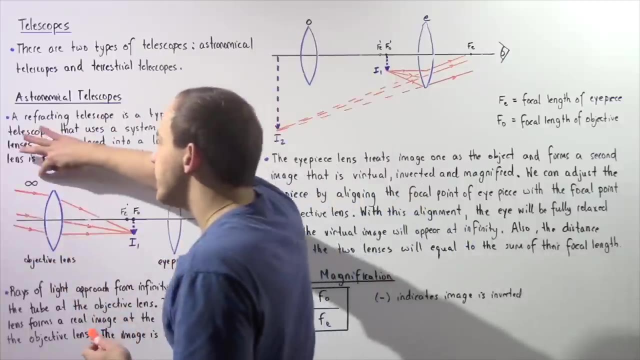 is the objective lens, and that lens essentially receives the rays of light from distant objects, planets, stars and galaxies. Now, because the distance between those planets and stars and this lens is very far away, we assume it's infinitely far away. Now, lens number two is known as the 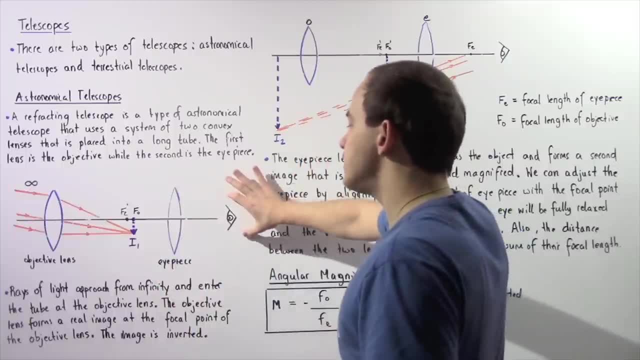 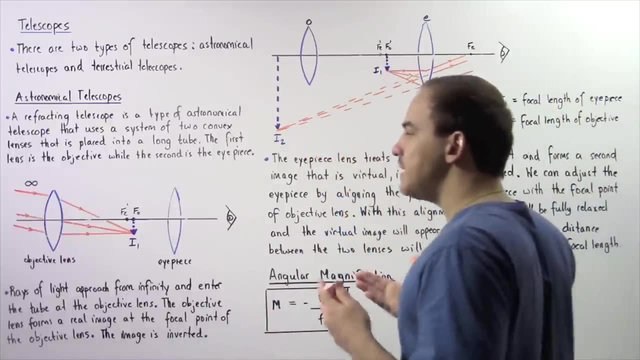 eyepiece lens. It's known as the eyepiece lens because this is where we put the eye when we hopefully get the eyepiece. Now, this is where we put the eye when we hopefully get the eyepiece. hold our telescope. Now let's examine what begins to take place when the rays of light hit. 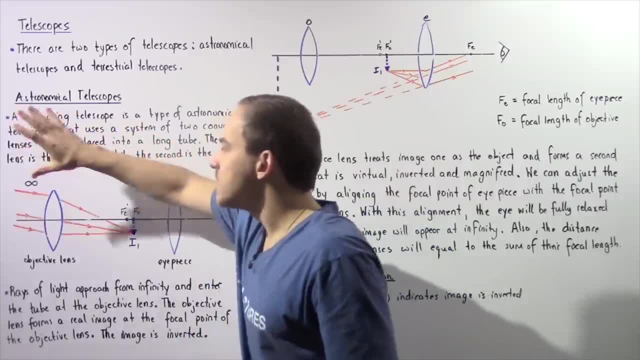 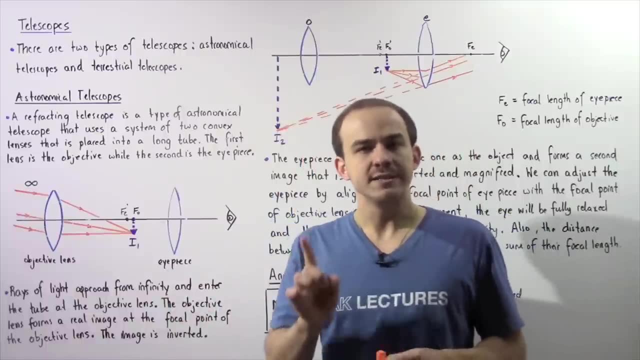 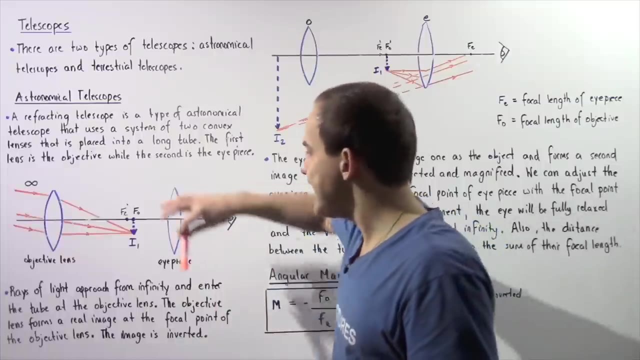 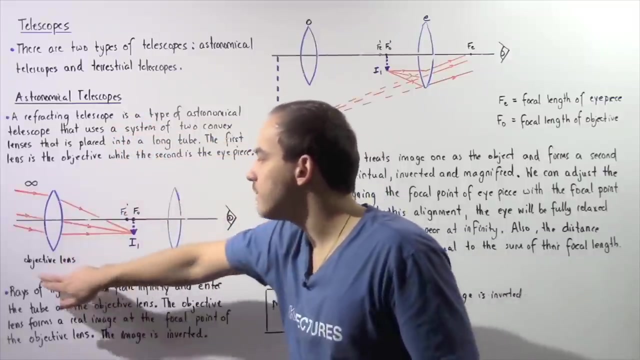 this convex lens Now, because the object distance is assumed to be infinitely large. that means, if we use the thin lens equation, we see that the image distance, the place where the image is formed, is equal to the focal length of that lens. Now FO is the focal length of the objective lens. 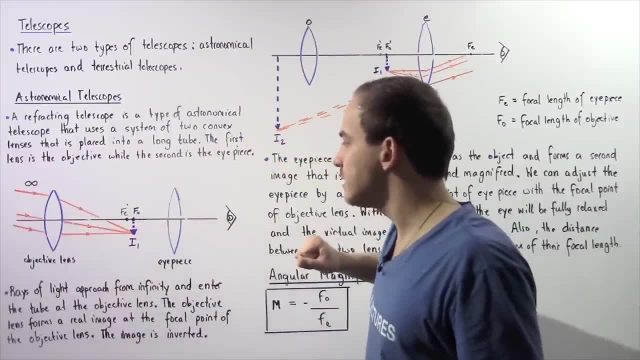 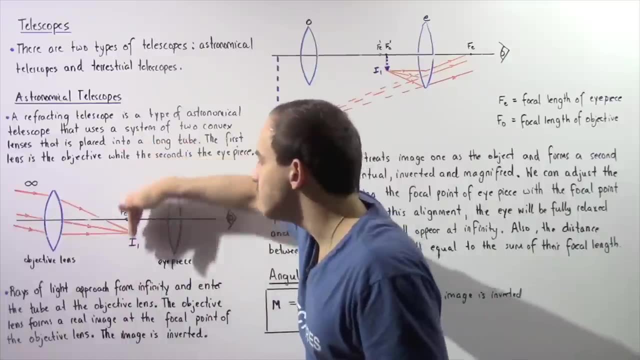 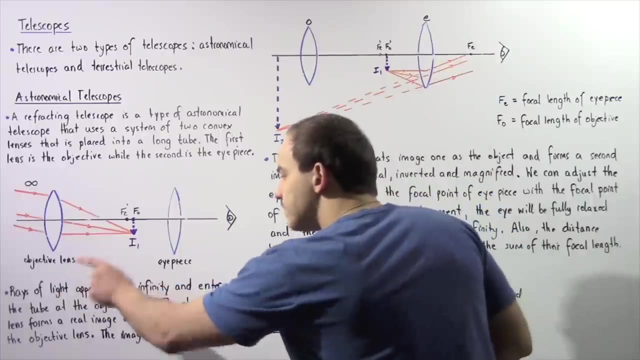 and FE is the focal length of the eyepiece lens. So that means the image that is formed by this lens will be located on the plane of the focal point of this objective lens. So the rays of light approach from infinitely far away is equal to the focal length of the lens. Now if we use 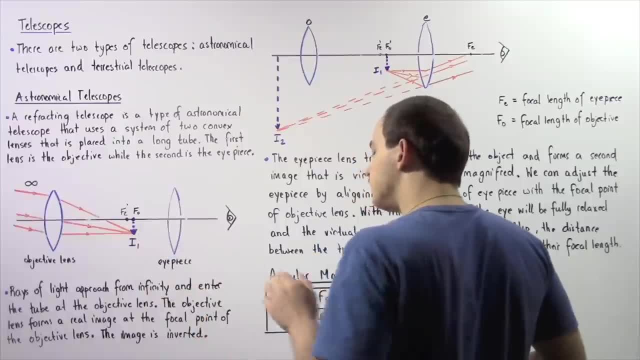 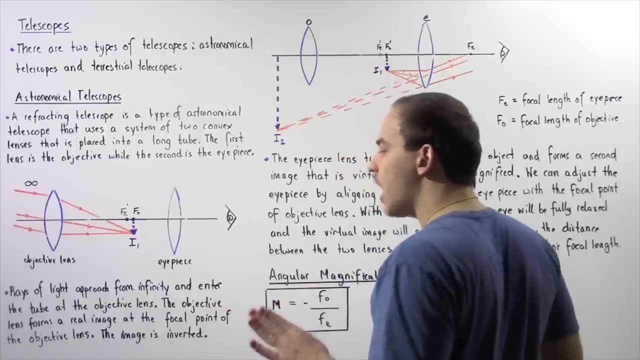 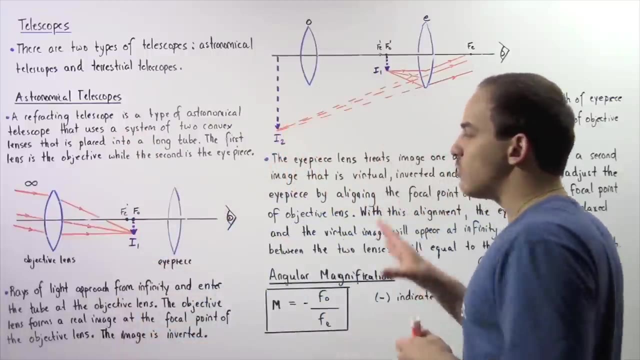 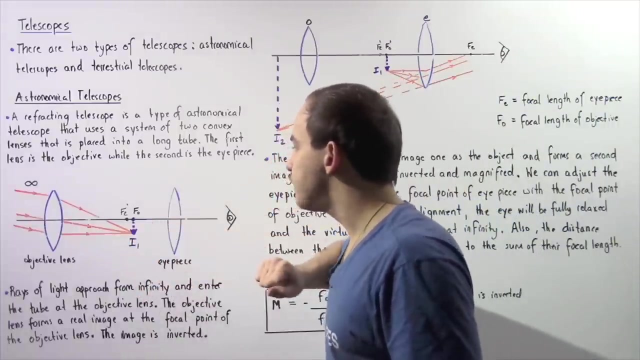 far away and enter the tube at the objective lens. The objective lens forms a real image at the focal point of that objective lens, at the, at the plane where the focal point is located. Now notice, the image is also inverted. So this is the image I1 that is formed on the plane of the focal point. 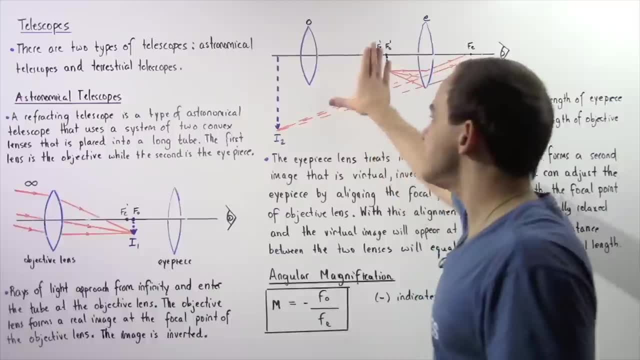 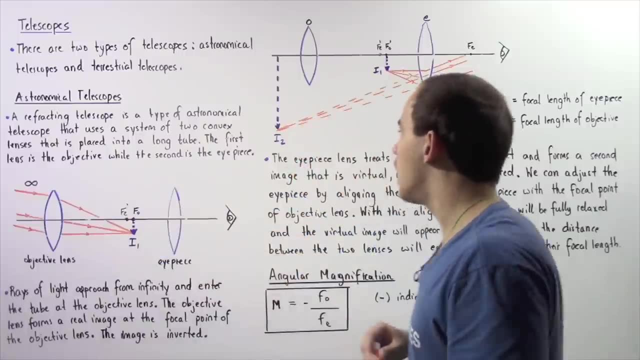 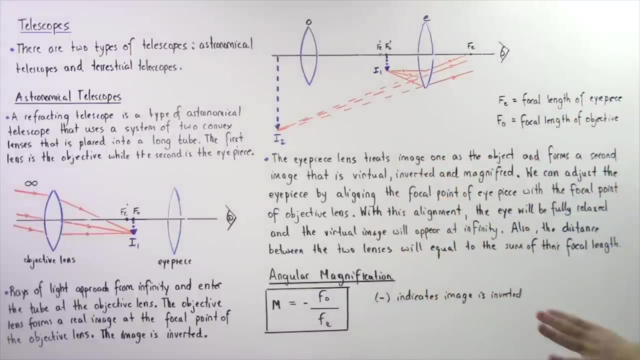 of the objective lens. So now let's examine what takes place. what exactly does the eyepiece lens do with this image I1.. So the eyepiece lens treats this image I1 as the object and forms a second image of that first image. and that second image is virtual, inverted and magnified as shown in the. 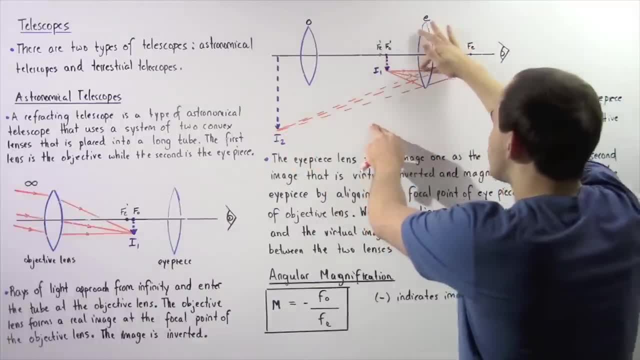 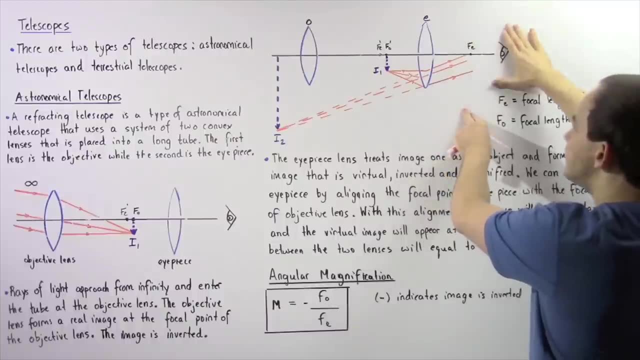 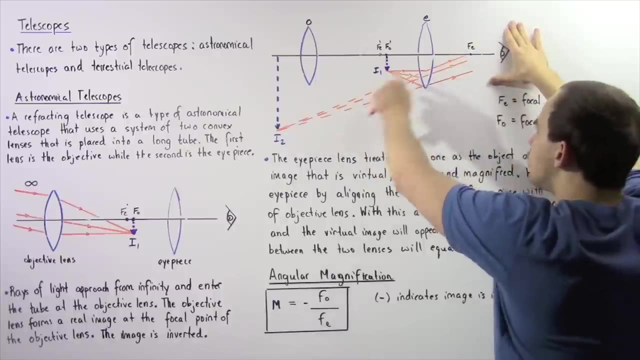 following diagram. So If we essentially observe these rays of light, these rays of light will essentially refract and will eventually end up at the eye of the person. Now, what the eye will see is these rays of light will essentially follow a straight path. and if we follow the straight path of these rays of light, 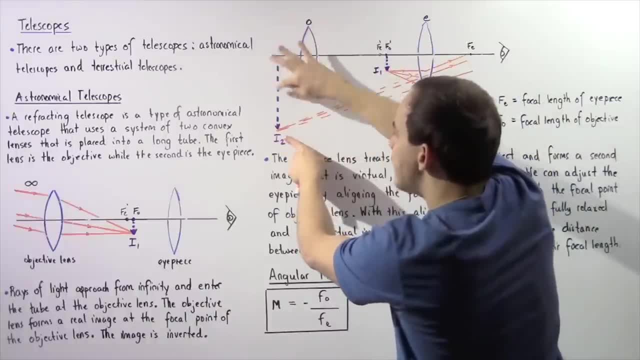 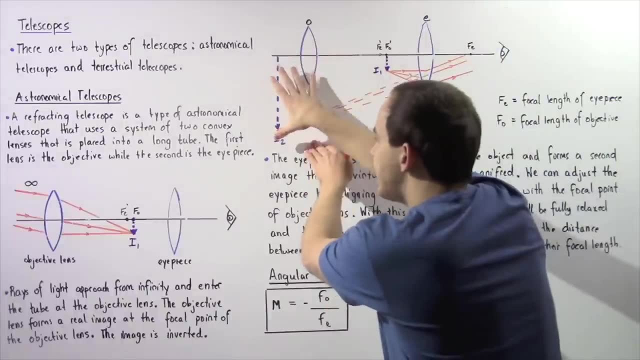 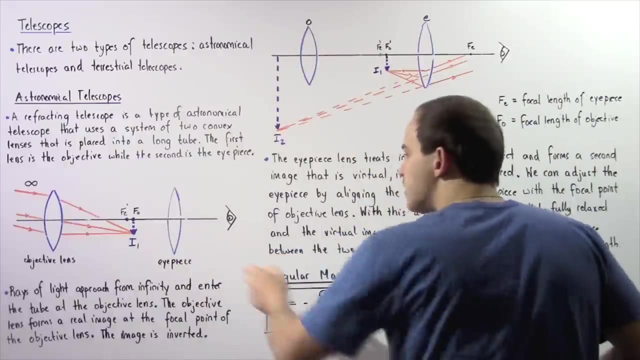 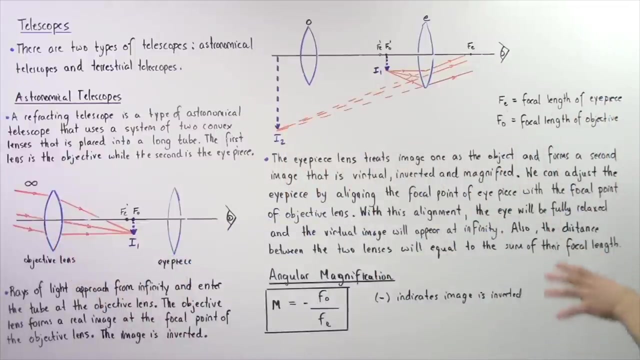 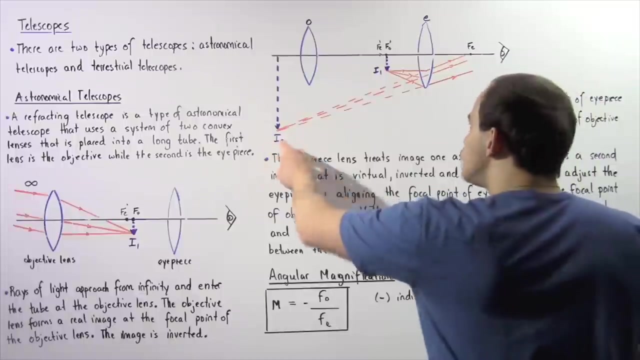 they will all converge at the following point and this will form our virtual image. image number two: and the eye. Should either皆 one see the face of the object or eye or the itself, And as one eye or eye becomes visual, the eye can also read this image. image number 2- and we will see. 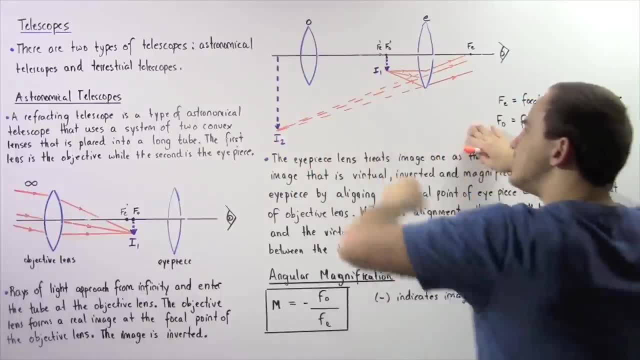 this image as if it was the object. So The eyepiece lens trees image, one that is formed by the objective lens as if it was the actual object, and forms a second image, The image Ugh, A virtual, inverted and magnified. so its virtual because it's found to the left of this lens. it's inverted because it points in the same direction, withild. 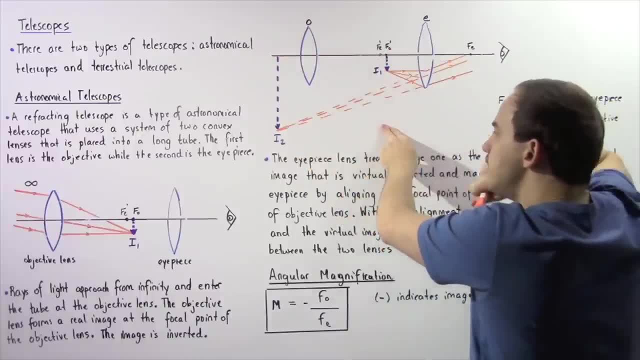 I sense there are Alexander Low warming in a number of parts, but this one, I1, a shadow that was important and known in the image field And that's why this image line, Lens, St Sound direction, as this image in the opposite direction, as the object, And it's magnified because it's 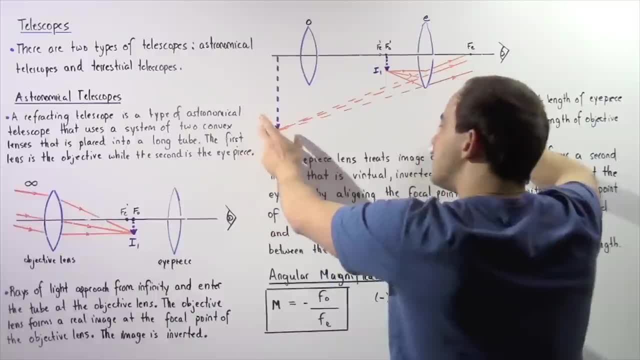 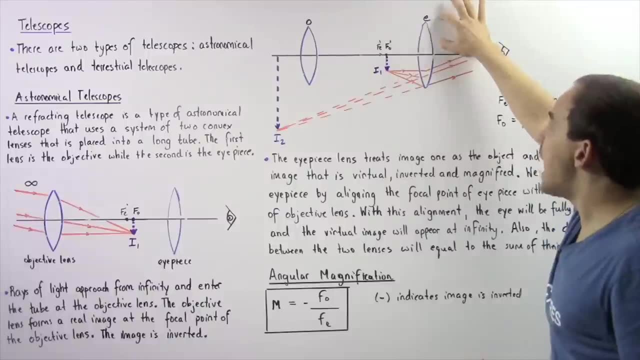 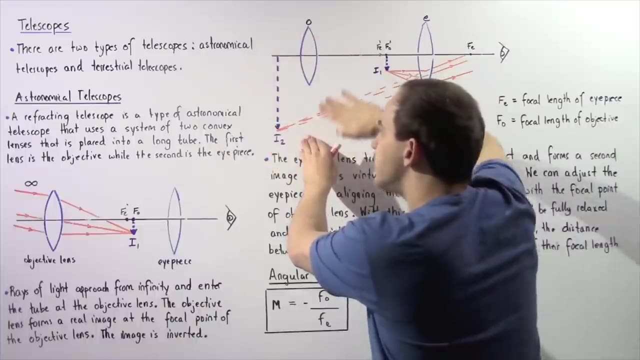 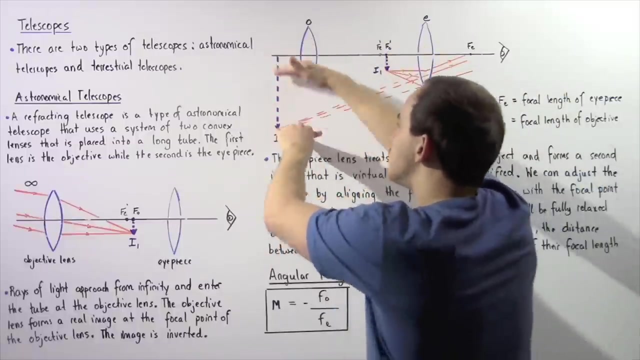 much larger than image one, So let's label this as image two. So, once again, image one is formed by the objective lens. the eyepiece lens forms image two and the eye actually sees this virtual image as if it was the object. So notice that it's much larger than image one and it's much 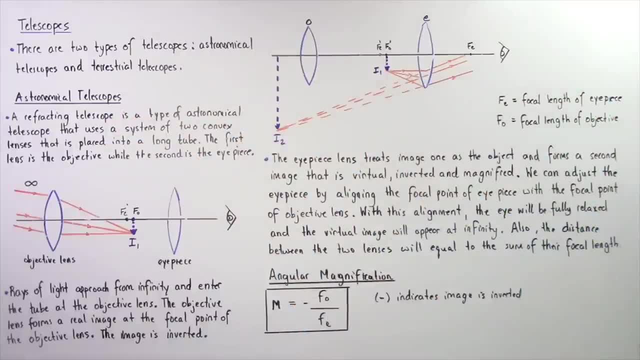 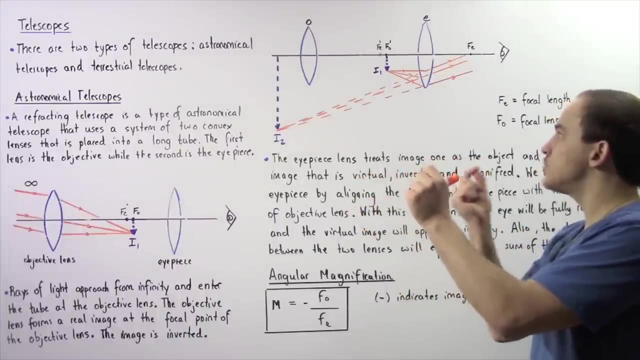 larger than the object that is seen by the naked eye. So we can adjust the eyepiece by aligning the focal point of the eyepiece with the focal point of the objective lens. So if we take our telescope, we can essentially adjust this distance so that the focal point of the 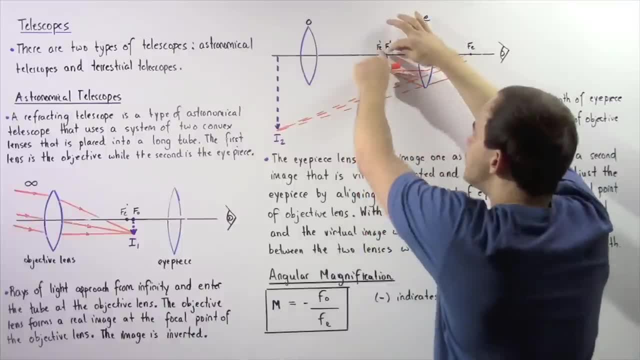 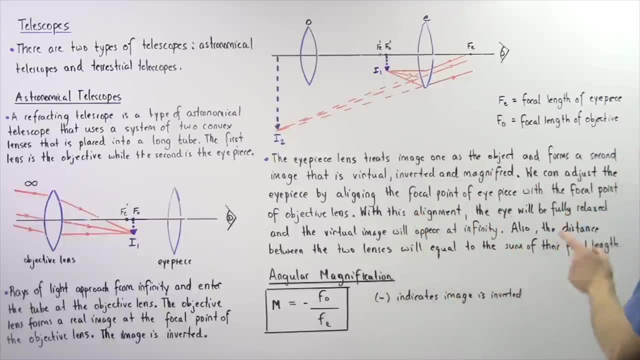 objective lens is much larger than the object that is seen by the naked eye. The objective is equal to the focal point of our eyepiece. So these two points essentially align. Now, with this alignment, the eye will be fully relaxed and the virtual image, this virtual image, 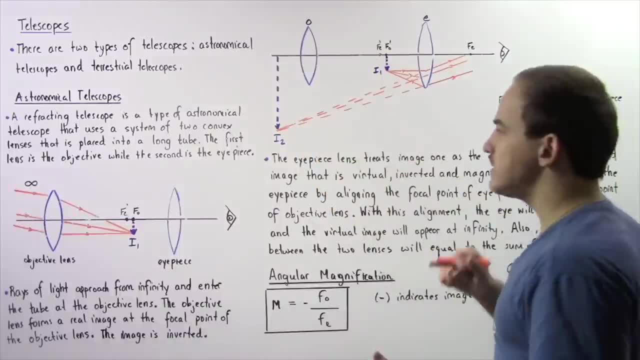 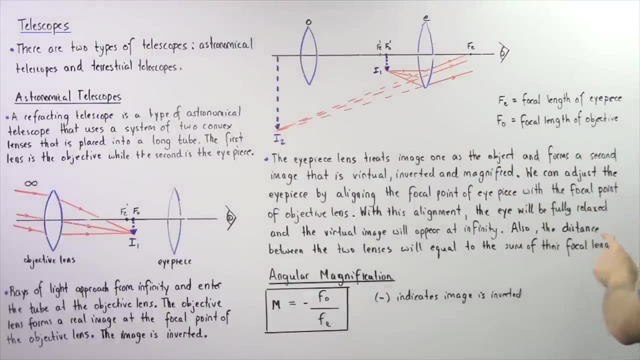 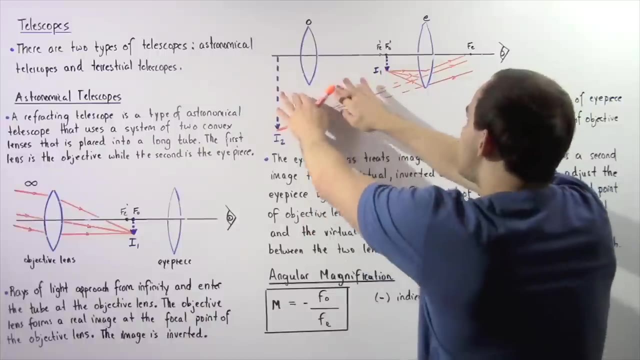 will appear infinitely far away. So that basically means it will be very large. Also, at this particular position, the distance between these two lenses will be equal to the sum of the focal length of the objective lens and the focal length of the eyepiece, That is. 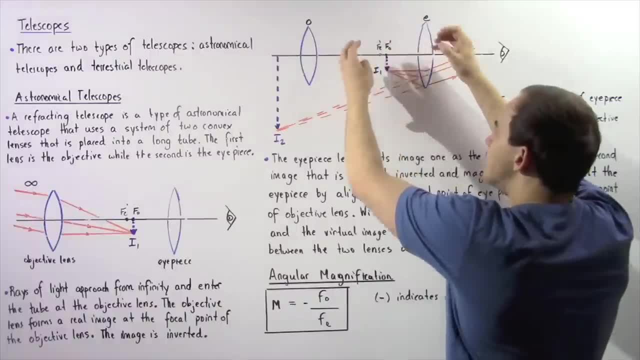 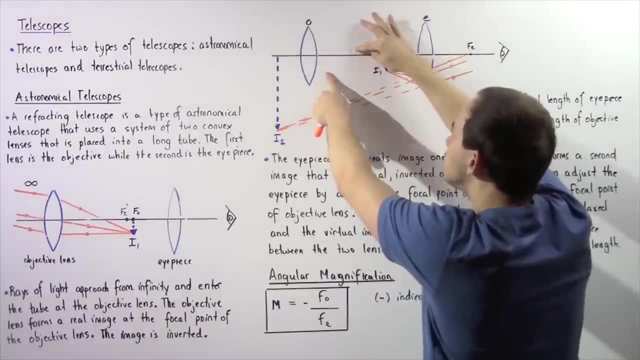 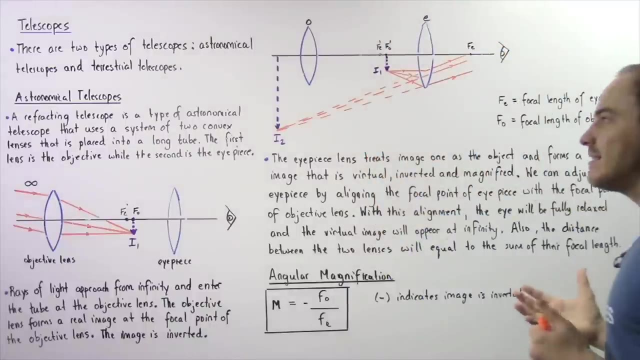 if we adjust this eyepiece so that these two points essentially intersect, that means this distance is equal to the distance of the focal length of the objective plus the focal length of our eyepiece. Now, what exactly is the magnifying power of a telescope? This is also. 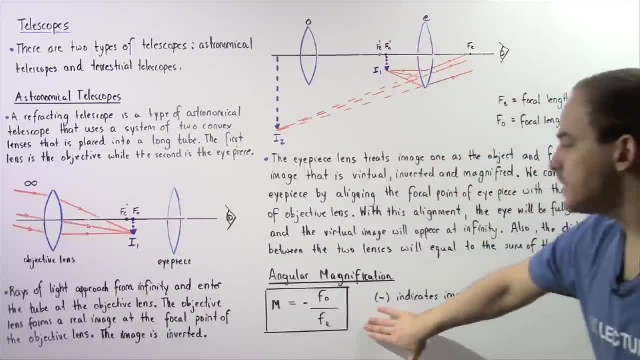 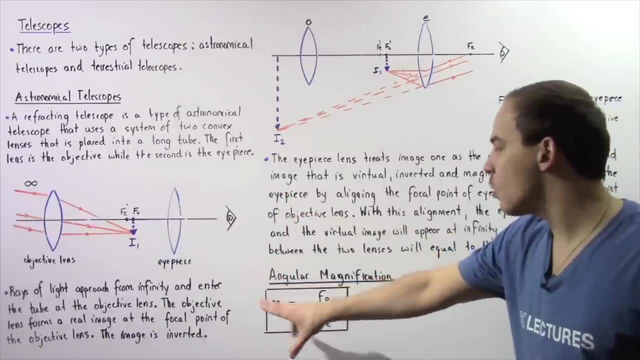 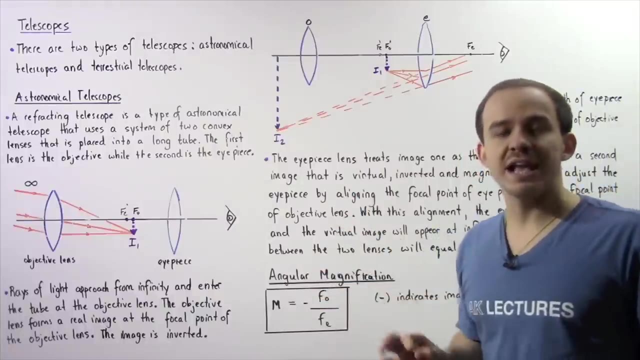 known as the angular magnification, and it's given by the following equation: So the angular magnification given by capital M of a telescope is equal to negative of the focal length of the objective lens divided by the focal length of the eyepiece. So notice, the larger our objective. 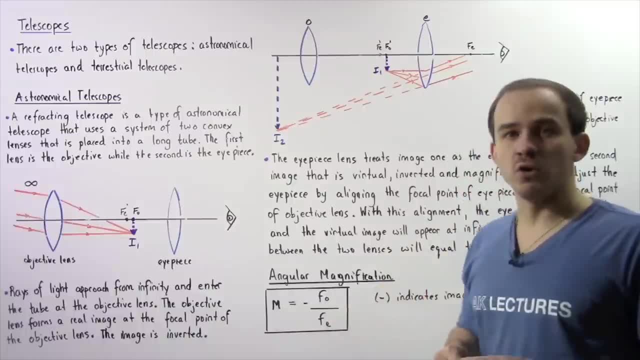 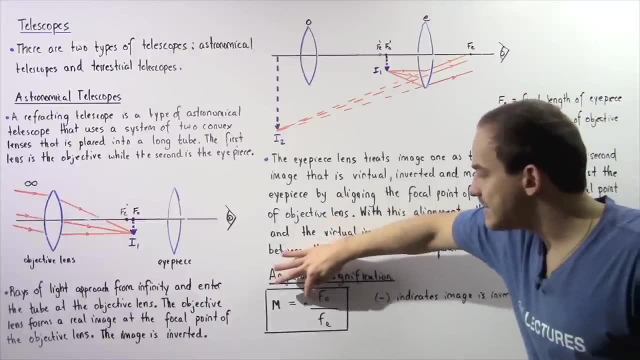 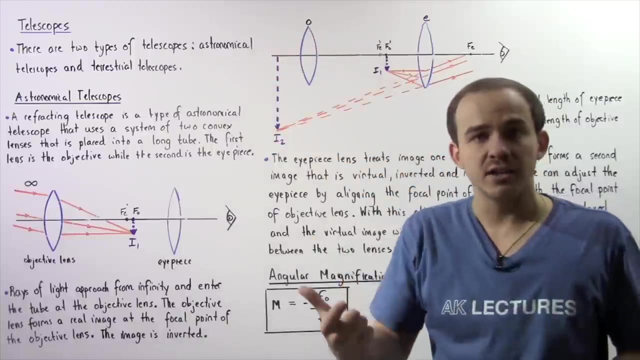 focal length is compared to our eyepiece focal length, the greater our magnification of our eyepiece, of our object is. Now, what exactly is the meaning of this negative sign? So notice, the virtual image is inverted and that's exactly why we place a negative sign. So this negative indicates: 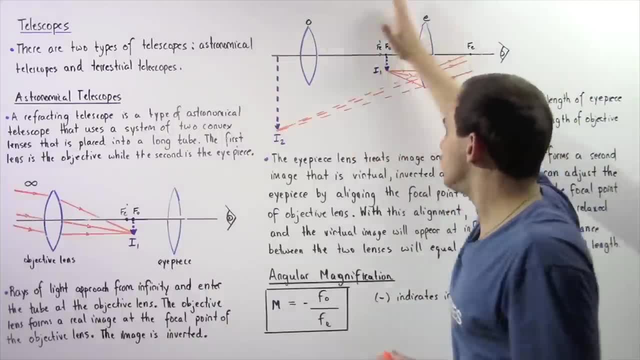 that the image formed by these two lenses is, in fact, an inverted image. 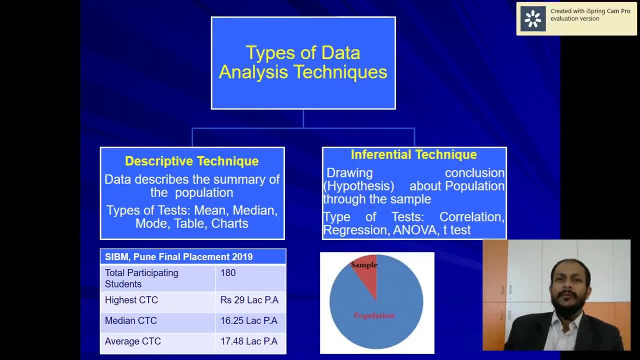 Hi, welcome to our channel talks on management and research. In today's session we are going to cover an important topic in research called type of data analysis technique. Broadly, we can classify the data analysis technique into two categories. one is descriptive techniques and another one is 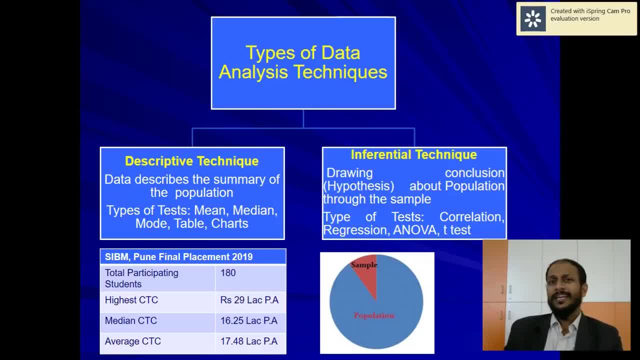 inferential techniques. These both comes under the category of two different type of statistical techniques that is predominantly used. Let us discuss it one by one Now. when it comes to the descriptive statistical technique, as the name suggests, it describes about the characteristics of the population or in. 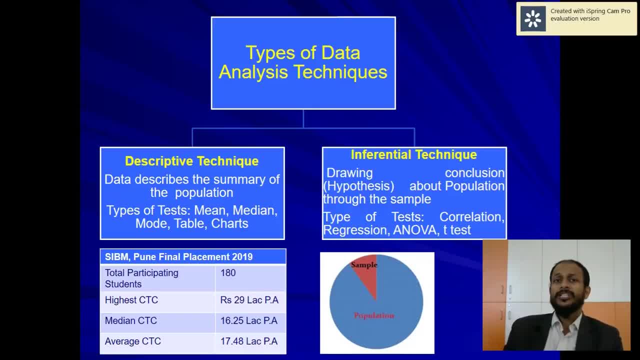 other words, whatever we are getting from the population, it used to represent it in a summarized form. Now we can have several kinds of techniques under this. we can use statistical technique to describe the characteristics of the population, or statistical test like mean median mode, charts, tables, all these. 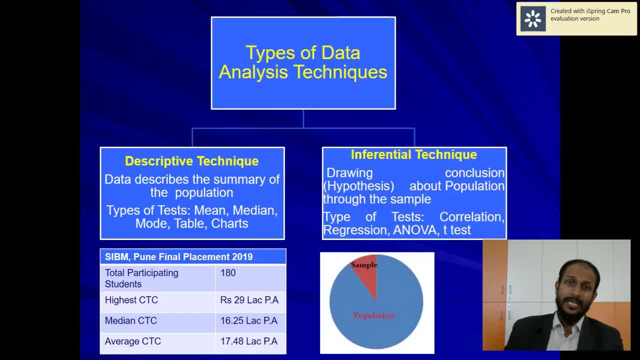 things comes under this classification of descriptive techniques. Here we don't take any particular sample of the population, but we take each and every unit of the population. Here we take a complete data set of the population and we give the entire characteristics of the population through the data that we 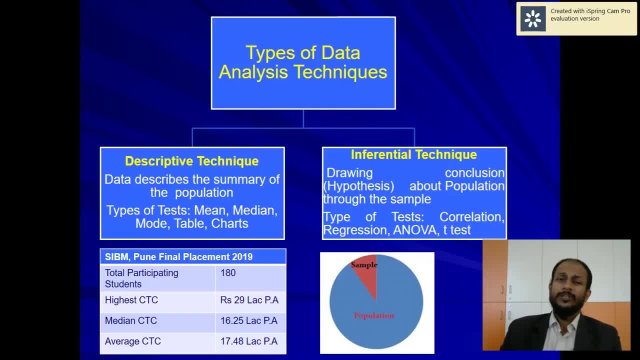 have obtained. Let me give you an example In this slide that you can see, I have shown you the placement statistics of SIBMB school in Pune, wherein you can see that almost 180 students have attended the placement, out of which you can see the highest placement figure is.